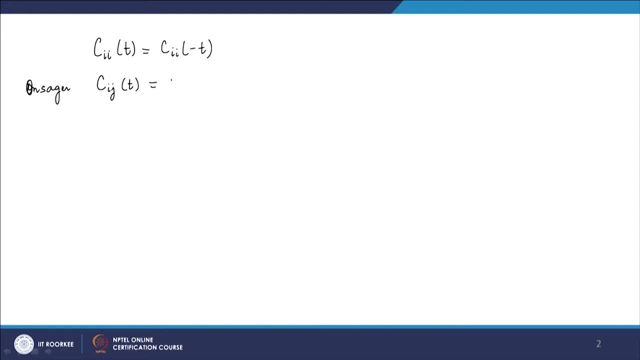 So the same property also holds for a cross correlation function. So just to recall, C ii is defined, C ii of time, t is defined as delta xi t, delta xi0, that is the same property. and C ij, t is defined as delta xi 0. 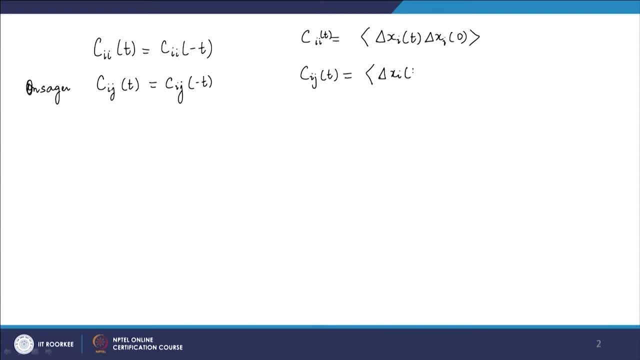 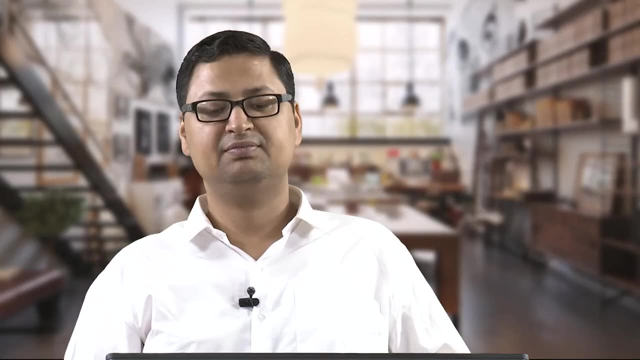 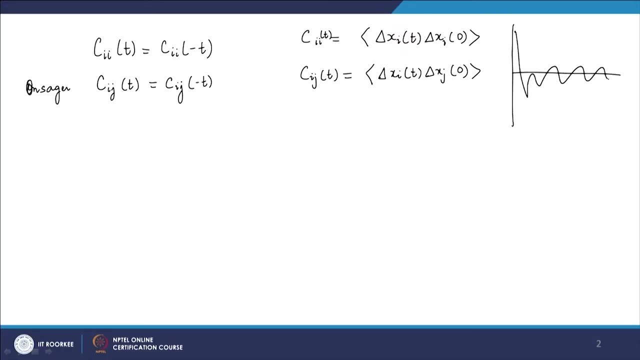 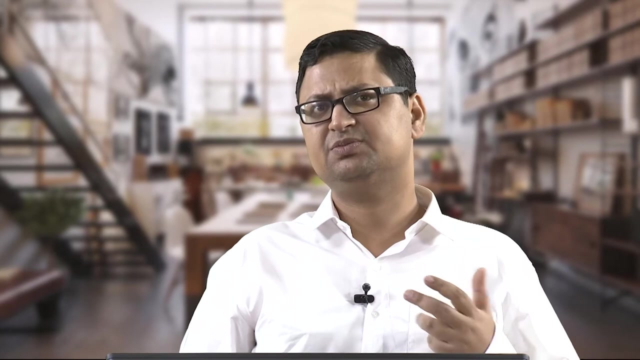 So C ii is defined as delta xi, t and delta xj 0. that is different property xi and xj, and both of them essentially fluctuate around a mean value, xi bar. So delta xi is the deviation from the mean value. So now there is a detail here that is not really of much concern to us, but it must be. 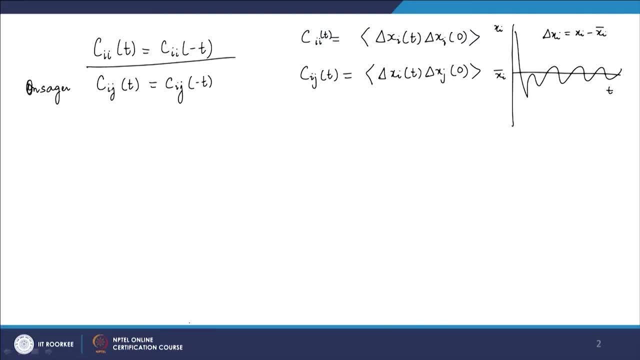 stated that although the first one is quite general, The second one only applies to properties that depend On positions and momentum of particle. this is true for the dipole movement that depends on the position of particles. it is actually true for many properties that only depends. 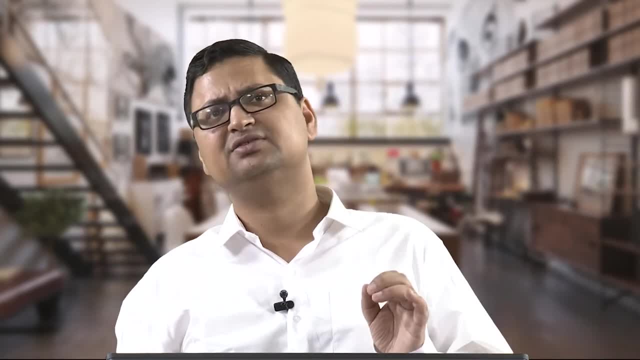 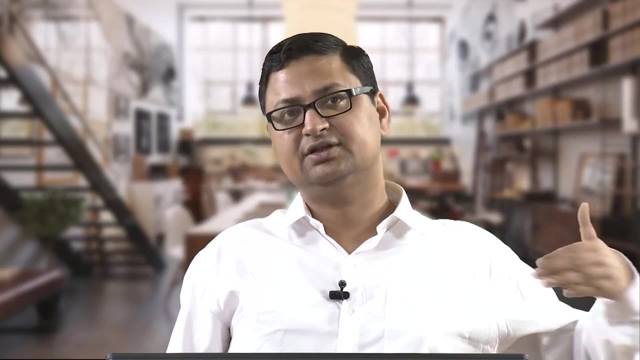 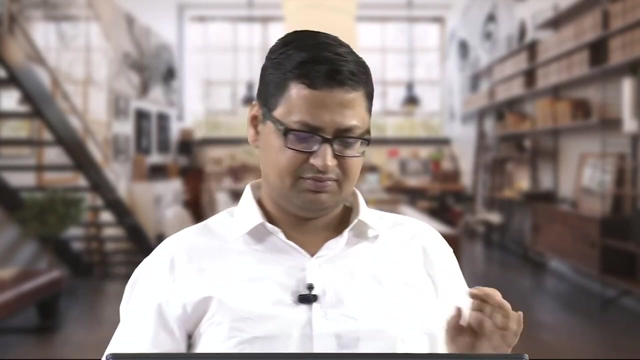 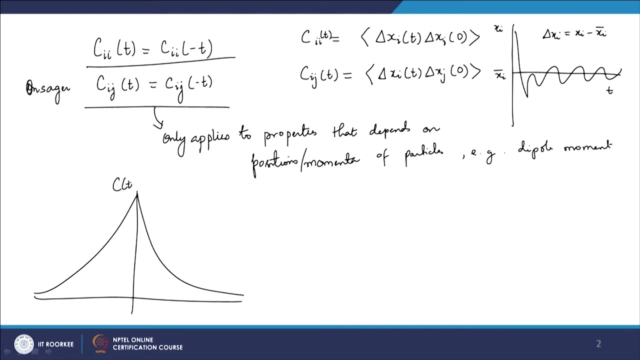 on position and momentum. It is not true for other properties that we typically do not care about In polymer physics, but you can read about the cases where this relation is not true. okay, So now what this evenness of these functions? so I am doing like Ct versus t. it is true. 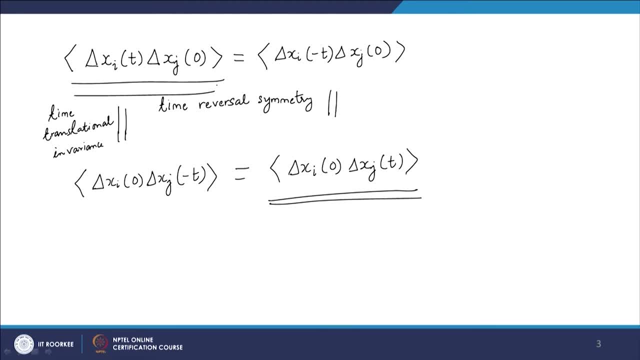 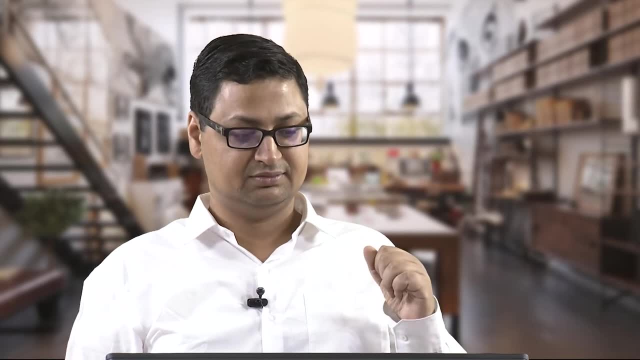 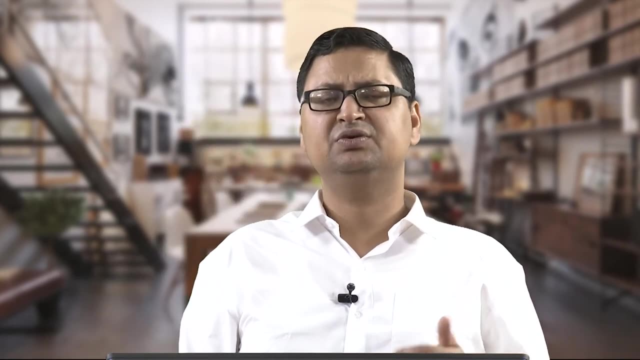 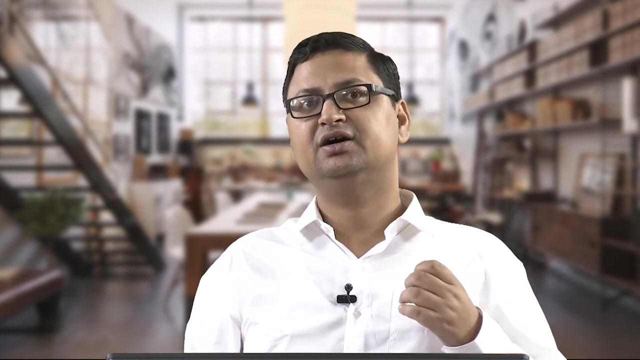 quantity. that is up there, okay. Now it turns out that instead of looking at just the autocorrelation or cross correlation in terms of the deviation from a mean value, it is sometimes more convenient to talk in terms of displacements instead of the deviation from a mean. let us say, if I am looking at 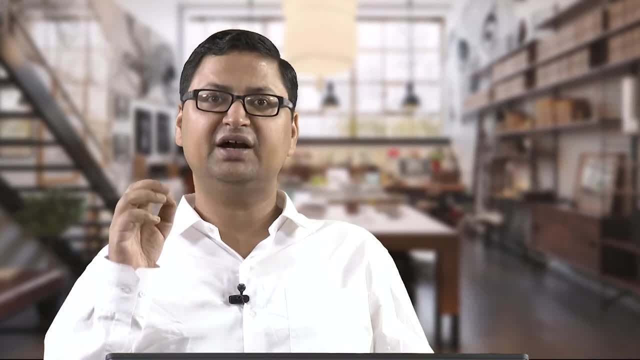 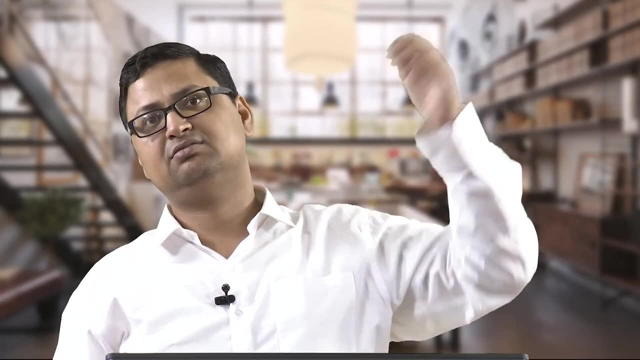 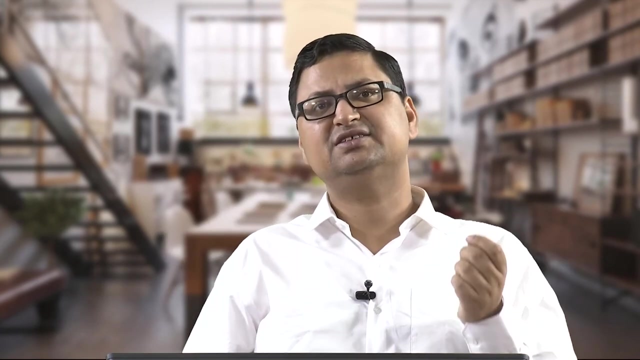 the position of a particular particle in the system. now there is no, there is a mean position. but the mean position can be like anywhere in the system. the mean position is not really constant for different particle in the system. What we can specify is the initial position and talk about displacements from that position. 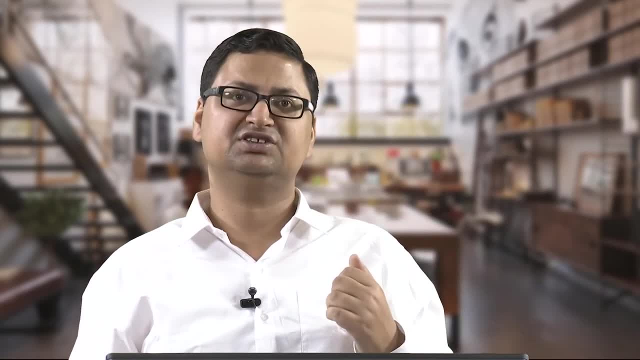 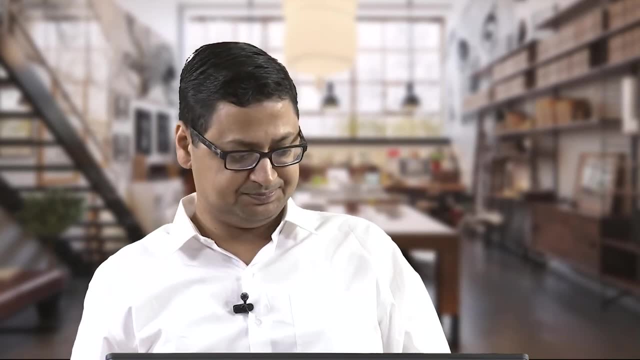 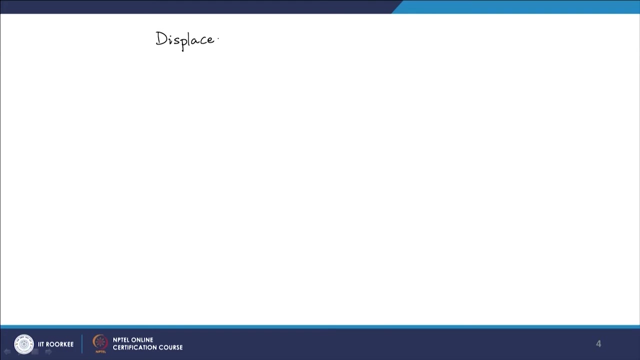 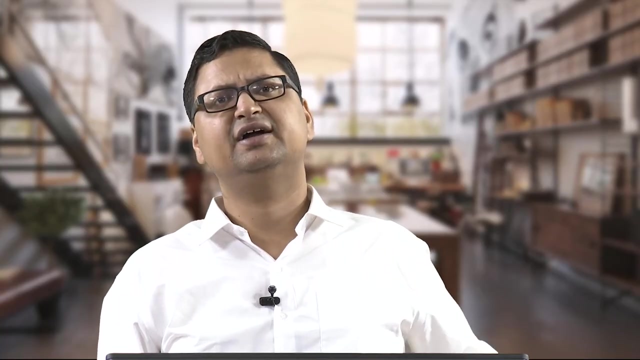 and in that sense we can define the displacement correlation function and which will become useful to us And what we will do next. so let me also define what is known as a displacement correlation function, which can be: So now I am not doing xi – xi bar, now I am doing xi t – xi at 0,. what is the displacement? 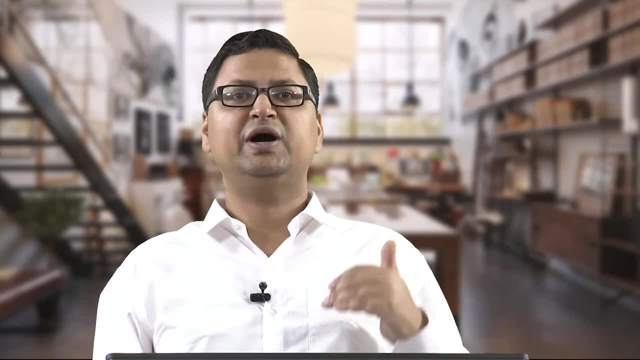 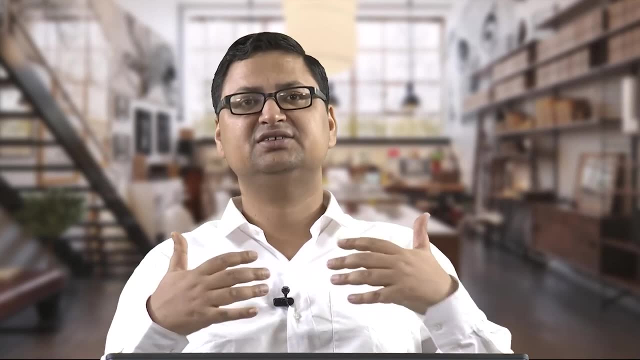 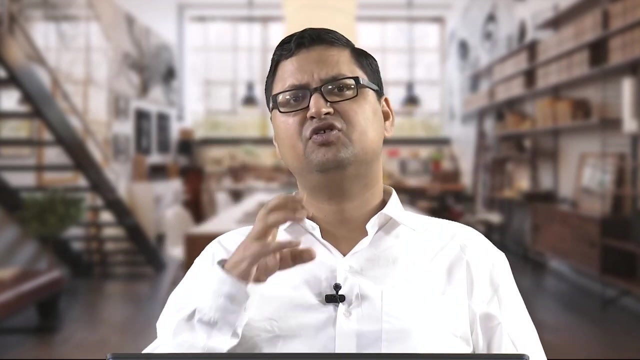 that has occurred from 0 to t. so although I talk about displacement, it should not always be in terms of like. only the length displacement does not have like a meaning in terms of dimension. it can also mean, for example, change in any property from an origin of time. 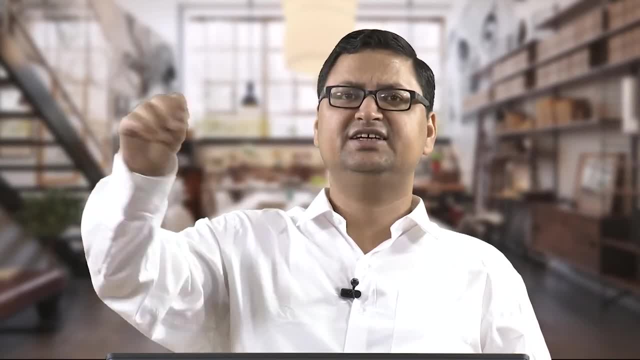 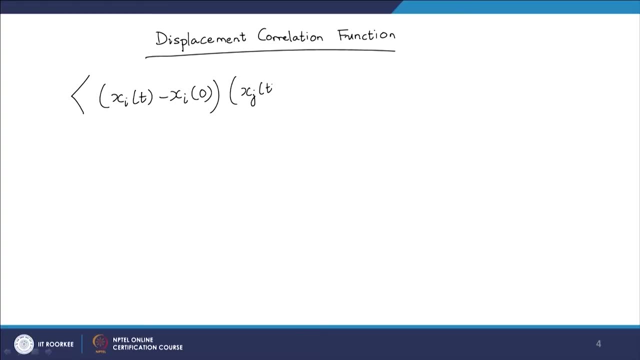 How much the property has changed, and that change is what I call displacement. so this I can also write in terms of deltas, because the mean values anyway will cancel out. so this will also be equal to. So if I expand this thing, What I get is delta XIT, delta XJT plus, delta XI0, delta XJ0 minus delta XIT, delta XJ0 plus. 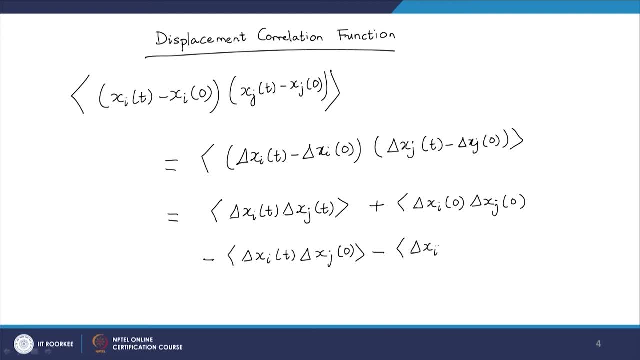 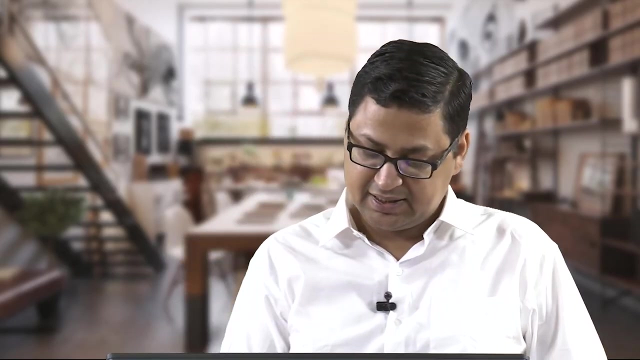 delta XI0 minus delta XI0 delta XJT. now, in this case, the first two terms are same by the time translational invariance, Since both of them are separated by 0, T minus T is 0 and 0 minus 0 is 0, and the last two. 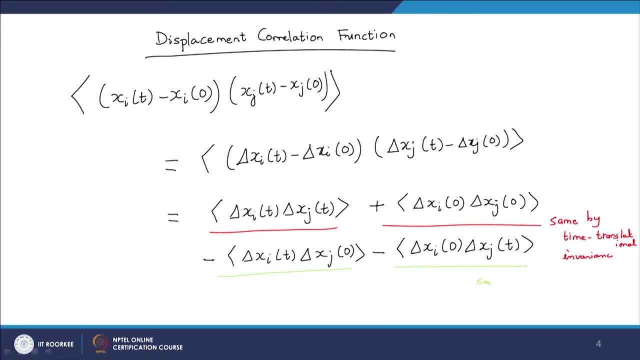 terms are also same by time reversal symmetry. so T minus 0 is opposite of minus T. so 0 minus 0 is 0 is 0.. So I get here: 0 is equal to 0, T is 0.. 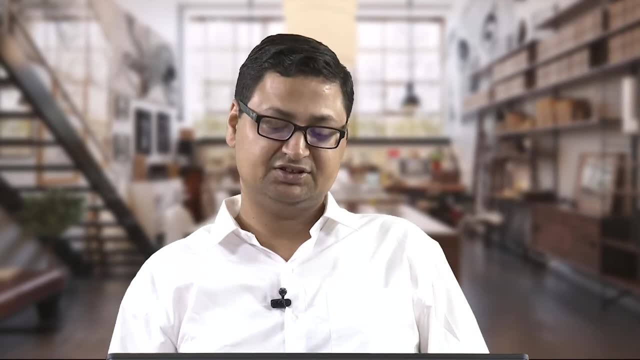 Here is what is равно 0. Hopkins is 0, 0 minus 0 is 0,. 3 is equal to 0, so equal number of addition, the total is equal to 0.. okay, So 1 into 1 plus one T. T divided by 0 times 0 is equal to 0. 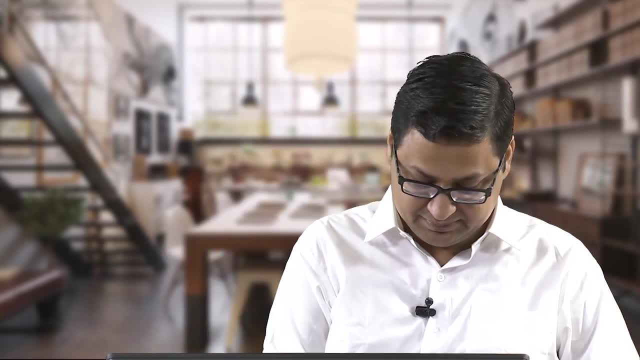 Let us assume that lambda is half. let us assume Alpha is half. 0 into minus 0. minus T is minus T. Actually, we use both time reversal symmetry and time translation invariance to get the second result. So what I get them is 2 multiplied by delta. XI0 delta XJ0 minus delta, XITR1 minus delta. 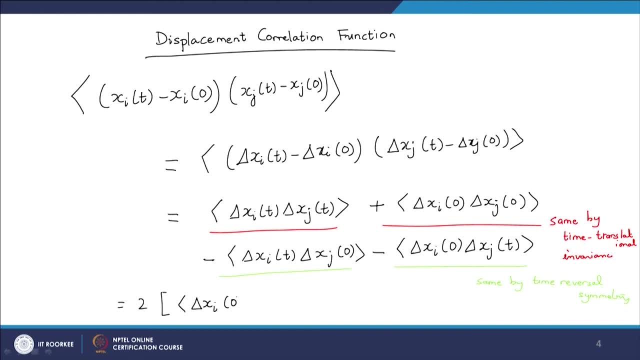 J0, R of X, 1 delta X1.. So that is the most fundamental decision we had made and we will be using this relation. we will use the relation that we have derived for the displacement correlation function later on. so please take note of this particular. 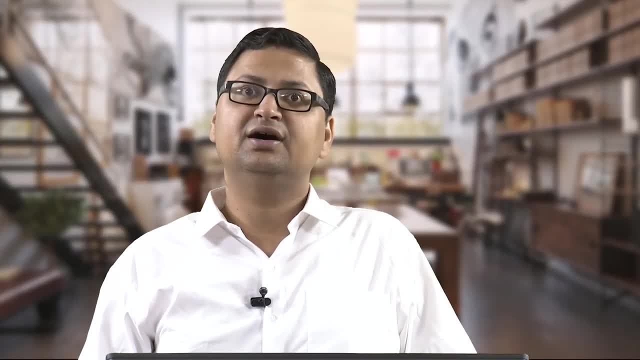 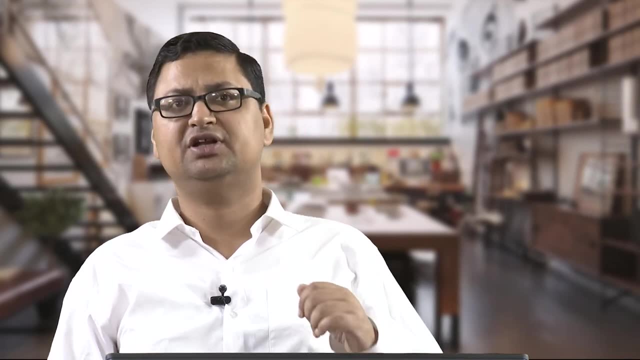 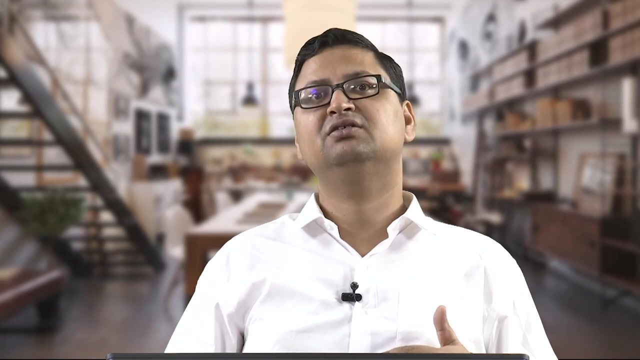 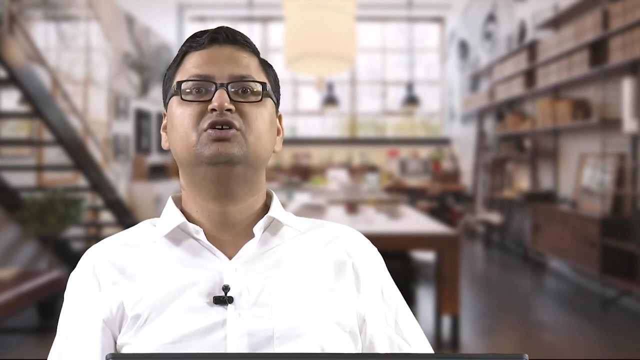 relation. So now, just like we can have a displacement correlation function, we can also talk about something like a velocity correlation function that would characterize the rate of change of position instead of position themselves. again, keep in mind that the system is still at equilibrium and we are talking about the motions because of fluctuations, not really. 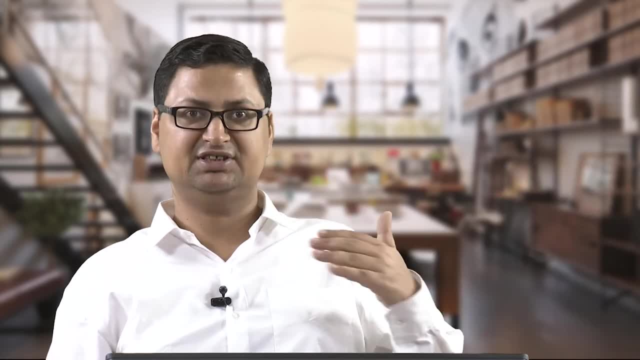 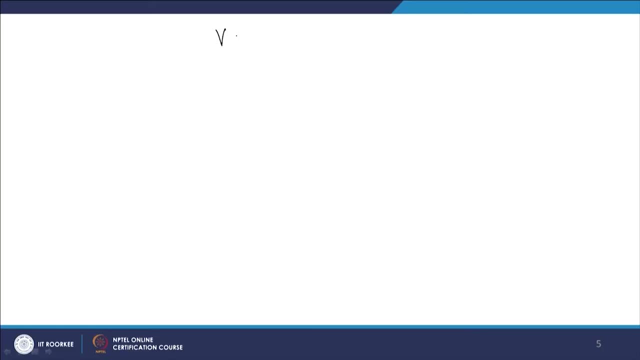 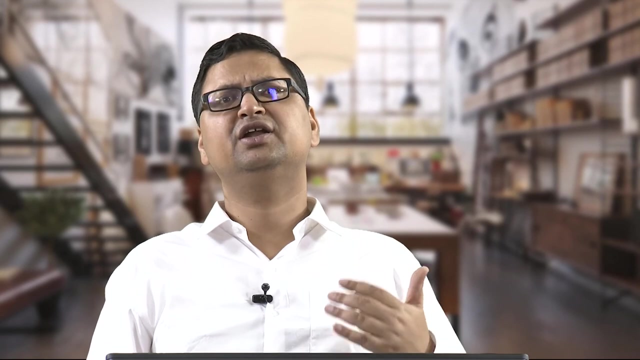 a bulk velocity for a system at non-equilibrium. in this case equilibrium is still holding, So we can also define the velocity correlation Correlation function. again, the velocity is the rate of change of any property with time, not really only the position with time. velocity is defined in a more general sense, so maybe 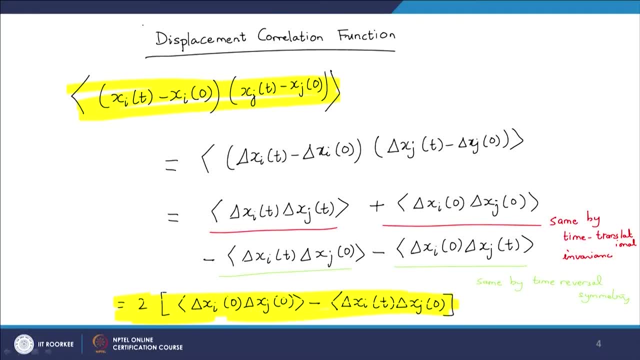 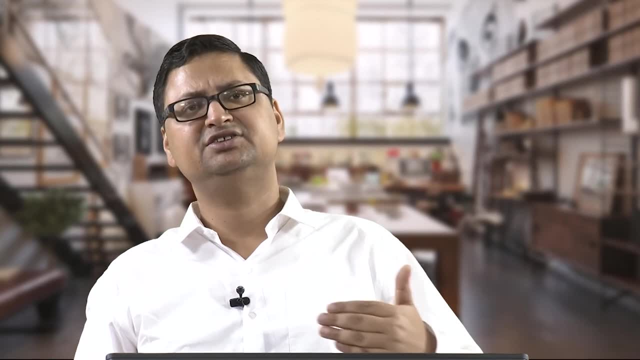 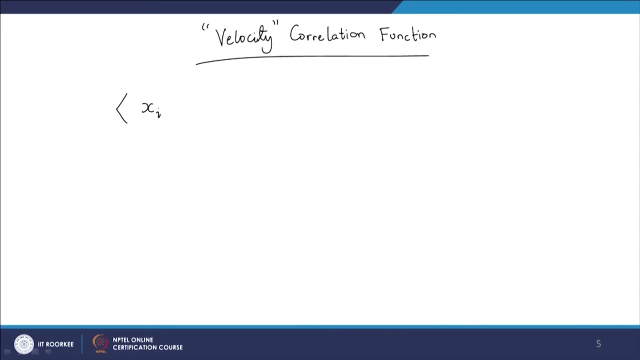 I will put the velocity under quotes, just like the displacement, Just to characterize that it is for any property, not really only for the change in position. so this I can define as xit, xjt, prime. that is the velocity correlation for i and j. so 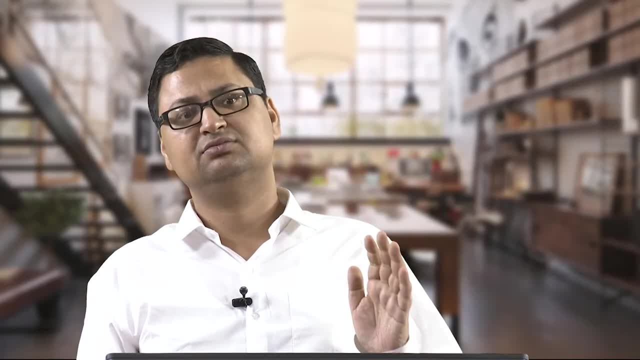 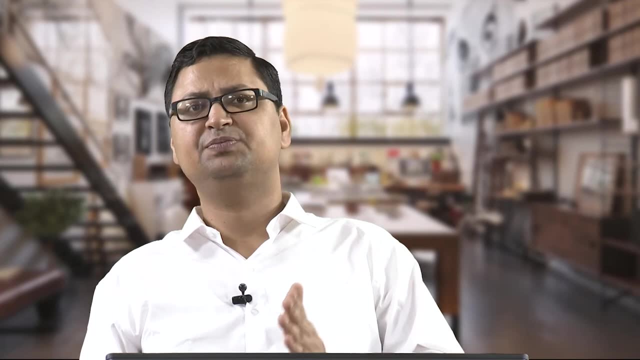 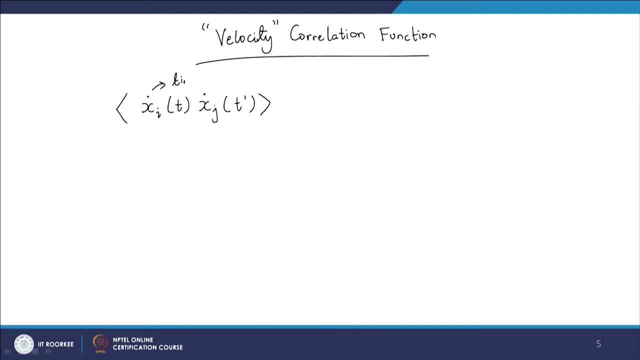 at time t and t prime. We have not yet said that this will also satisfy the time transition invariance, so we have written in terms of t and t prime. So now: and dot represents the time derivative. So now this I can write as: . . .